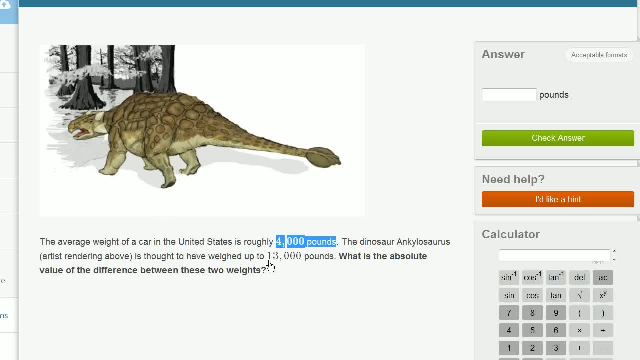 The dinosaur Ankylosaurus artist rendering above is thought to have weighed up to 13,000 pounds. What is the absolute value of the difference between these two weights? You could calculate the difference between these two weights. You could take the smaller and subtract from the larger. 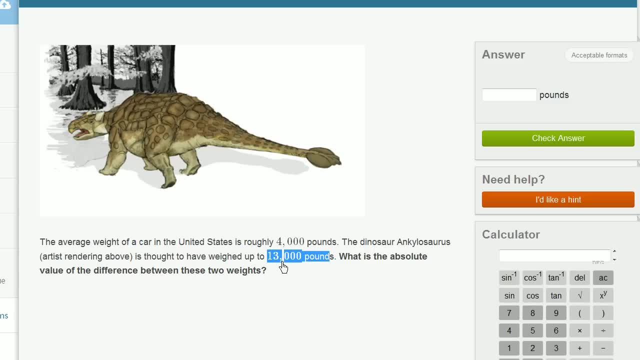 so if you take 4,000 from 13,000, the difference would be 9,000 pounds. The absolute value of 9,000 pounds is 9,000.. You could have gone the other way. You could have subtracted 13,000 from 4,000,. 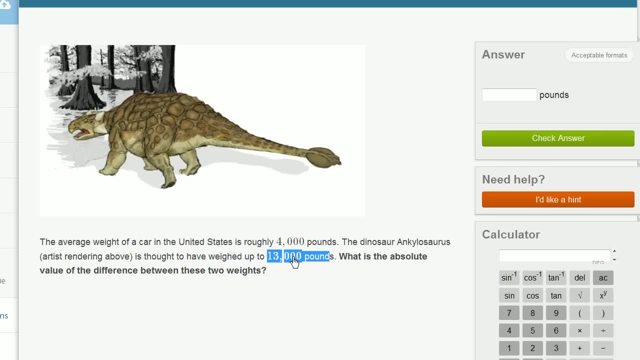 and you would have gotten negative 9,000, but the absolute value of negative 9,000 is still 9,000.. We just want to think about the absolute difference between these two. We don't want to think about which one we're subtracting from whichever one. 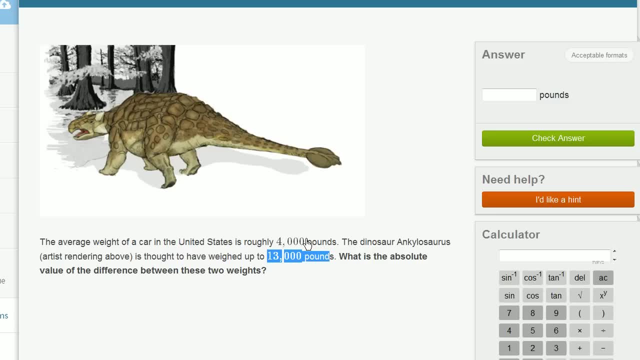 Whatever we're subtracting from the other one, we just find the absolute difference. Whether the difference was negative- 9,000 or 9,000, depending on which one you subtract from the other, the absolute value of either of those is going to be 9,000 pounds. 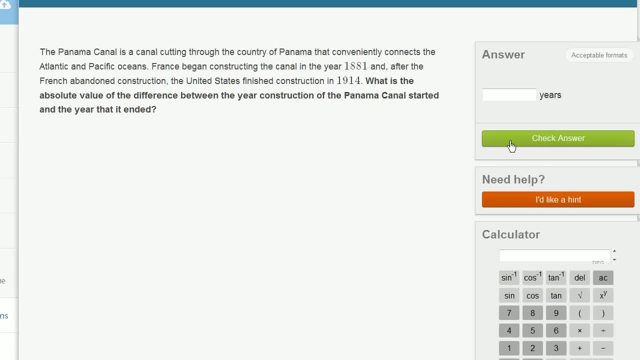 9,000 pounds. Let's do one more. No picture this time. I was getting used to that. The Panama Canal is a canal cutting through the country of Panama that conveniently connects the Atlantic and Pacific Oceans. What's nice about these is we learn other things. 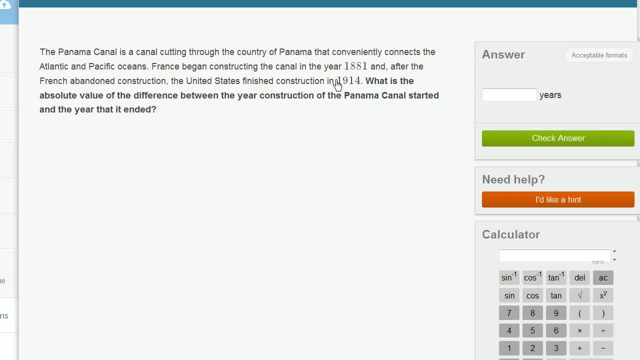 other than mathematics here. France began constructing the canal in the year 1881, and after the French abandoned construction, the United States finished construction in 1914.. What is the absolute value of the difference between the year construction of the Panama Canal started? 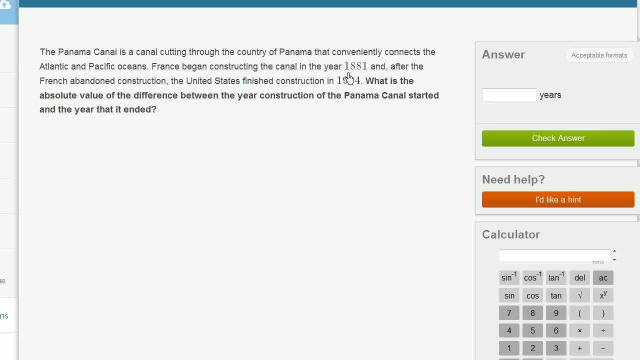 and the year that it ended. Well, you might want to, just if we just did it the way that they. well, there's a couple of ways you could do it. You could take the larger year and subtract the smaller year from it. 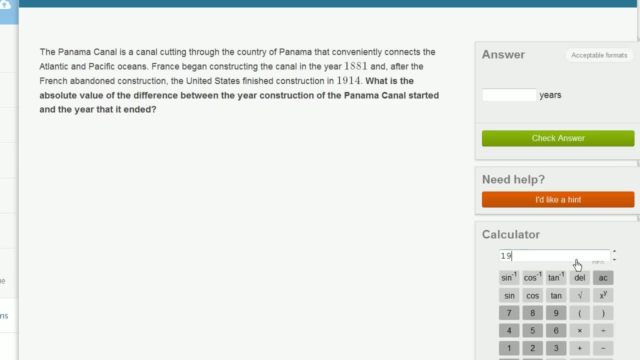 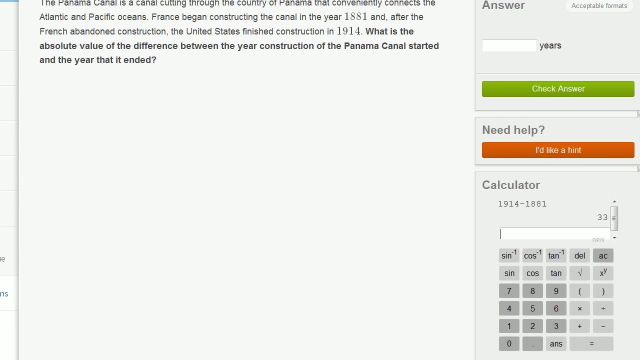 We have our calculator here. You could literally say 1914 minus 1881, and you get 33 years, And the absolute value of 33 is just 33.. Or you could have done it the other way around, Since we're taking absolute value. 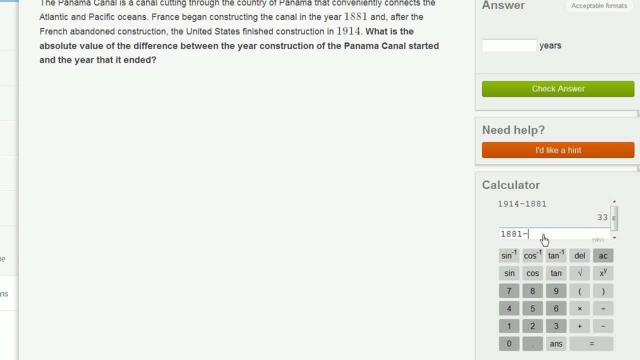 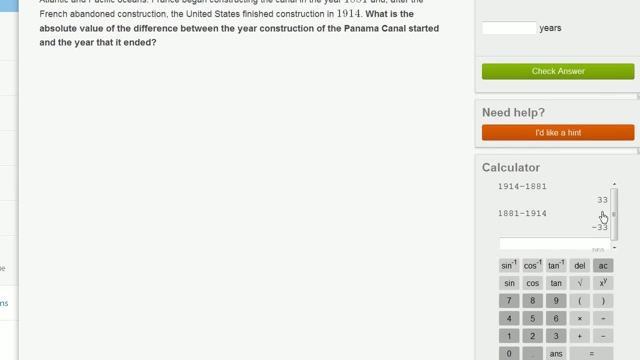 it doesn't matter what we subtract from the other ones. You could do it on 1881.. Minus 1914, and you would have gotten negative 33.. But the absolute value of either of these numbers is you're saying: how far is 33 or negative 33 from 0??